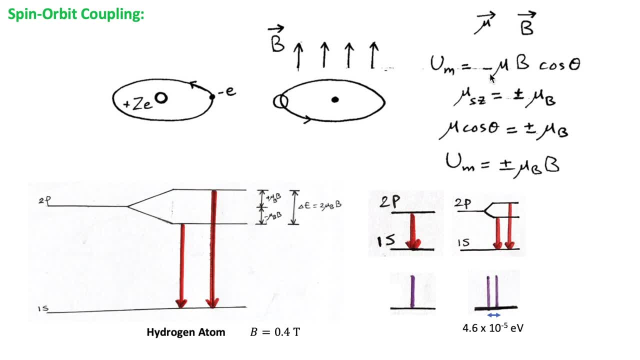 vectors. so this quantity, mu, cosine, theta is the, is the component of the vector mu that is parallel to b. okay, and in the case of the spin orbit coupling we have a vector mu that is parallel magnetic moment of the electron. this component is given by mu s z equal to. 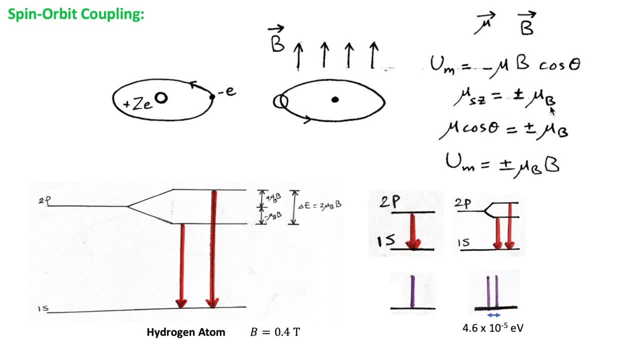 plus or minus mu B, where mu B is born magneto. so details of this can be found in the previous lectures I have given about quantum physics. so mu U M is equal to plus or minus mu BB. so depending on the orientation of the spin vector s, the energy of an atomic electron is either higher or lower by. 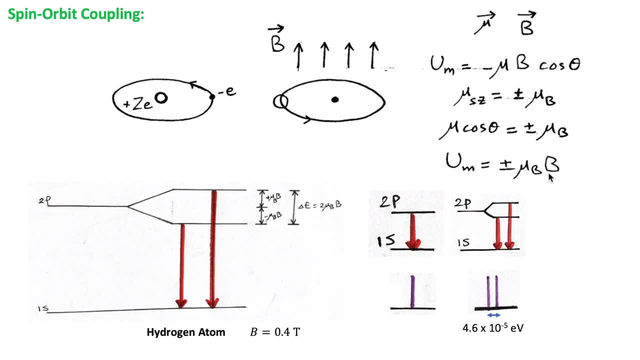 this quantity, which is mu BB, then in the case when there is no spin orbit coupling, so this is the 2p state, but but this is the actual states that correspond to this level when spin orbit coupling is taken into account. okay, so the result is that every quantum 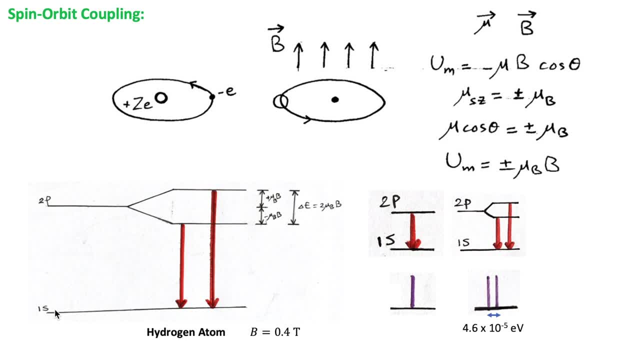 state except s states in which there is no orbital angular momentum, is split into two substates, and this is known as fine structure doubling. so the value of the spin quantum number s equal half is the only one that agrees with the observed fine structure doubling, and this is because, with spin the single, 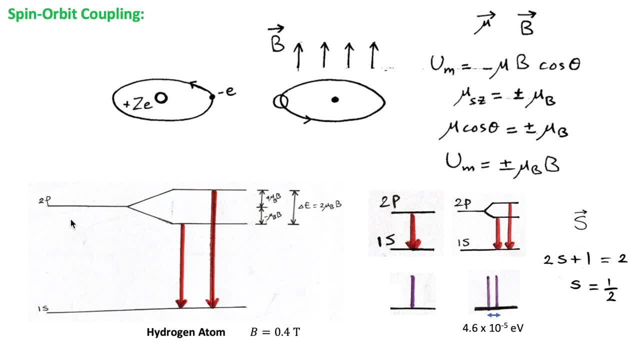 state is actually twin states. okay, so each single state, except for the s states, is actually two states, and the number of possible orientations of the spin vector s is equal to 2s plus 1 must be equal to 2, right, because we have two states and this gives the spin quantum number equal. 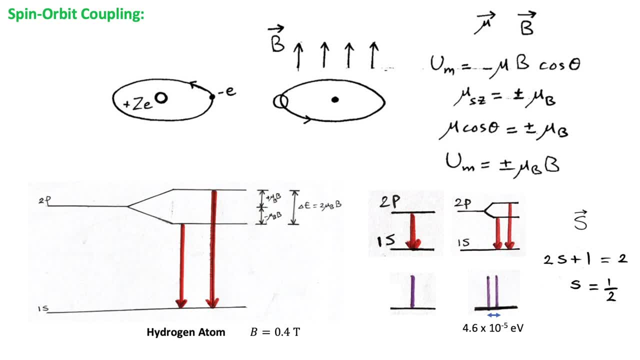 to half, so we can calculate the, the approximate magnetic field expression, which is equal to zero, and the number of possible orientations i have mentioned here as well. so this is: the f applied by f is equal to 5.. Now if i were to substitute it with the f of the hydrogen atom, and this will result: